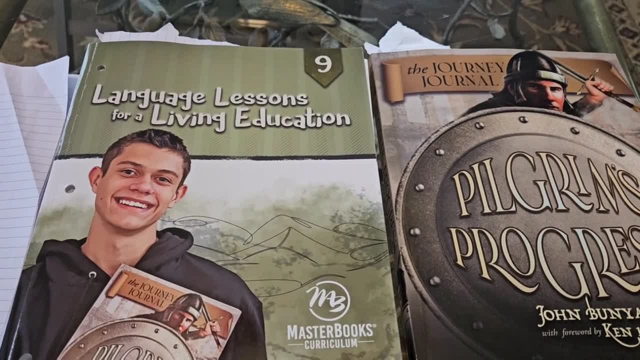 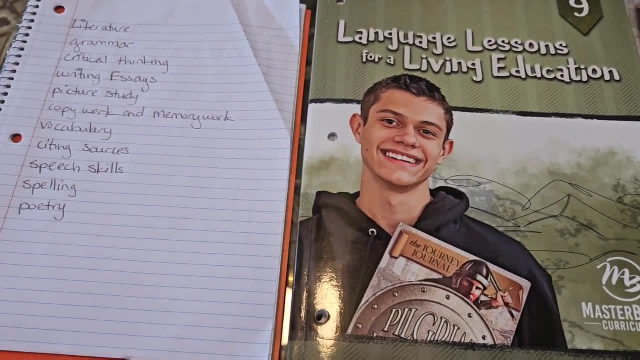 Hey guys, my name is Sandy. I'm a homeschooling mom to two boys. They're going to be going into 9th grade and 11th grade next year And this is our 8th year homeschooling, or it's going to be. 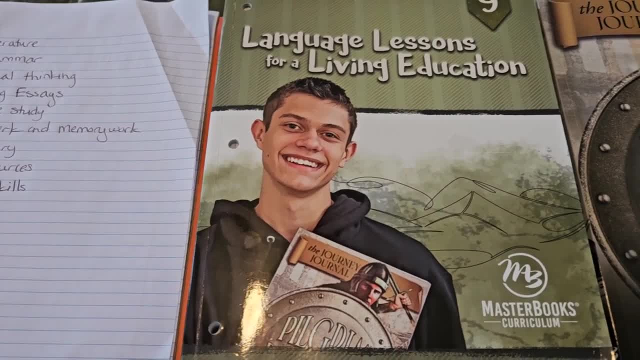 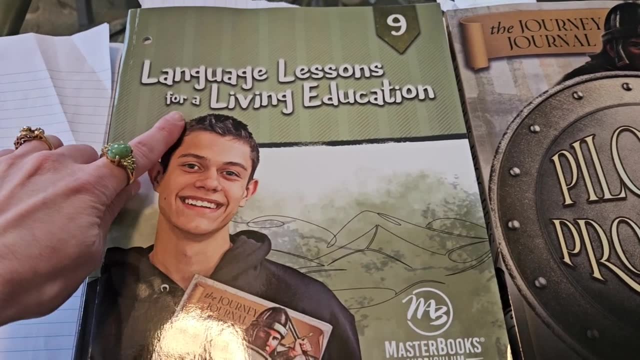 our 8th year homeschooling next year. This is my second child to go through the language arts in 9th grade And this is what I've chosen for him to use next year. It's Language Lessons for a Living Education from Master Books. This is a brand new curriculum they just came out with a few months. 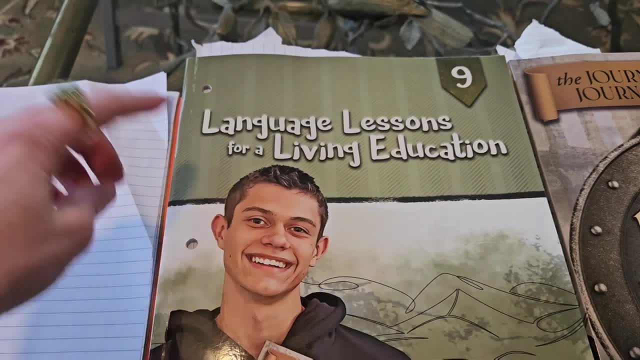 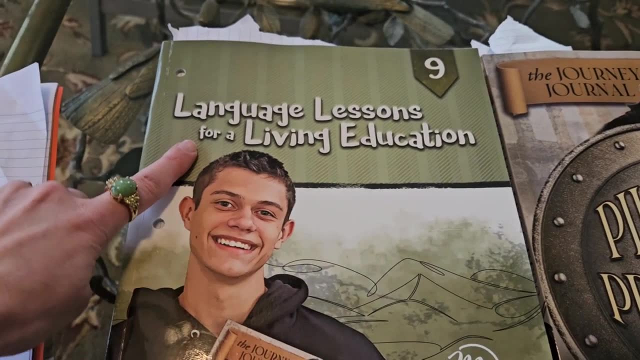 ago. He has actually used Language Lessons for a Living Education in the past. I believe it was for 4th or 5th grade, And he did enjoy school that year a lot, So I've selected this. I think it's going to be a great year for him. This is everything, just from looking over the textbooks. 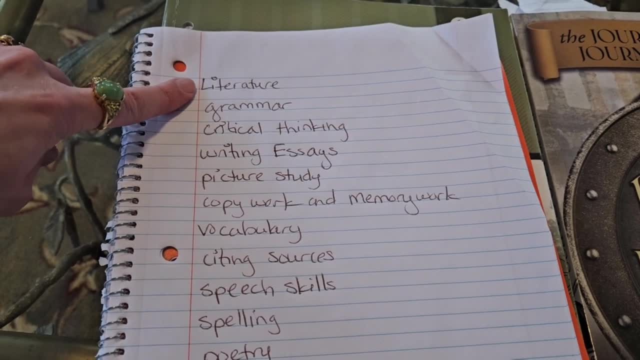 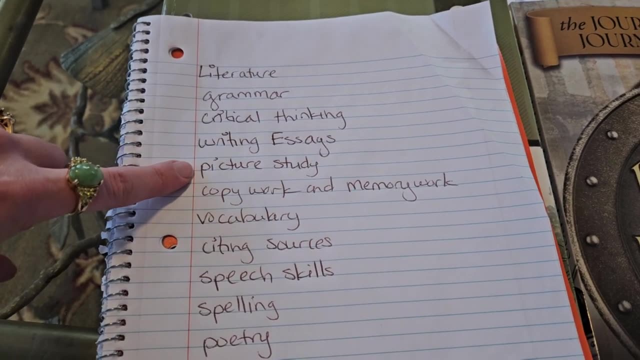 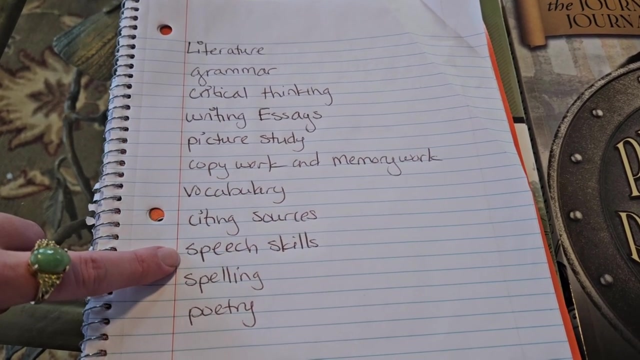 that they cover Literature. They only cover partial literature, so you need to add more to it. Grammar, Critical Thinking, Essay Writing, Picture Study, Copywork and Mathematics, Memory Work, Vocabulary, Citing Sources, Speech Skills, Spelling, Poetry. Now on the spelling. 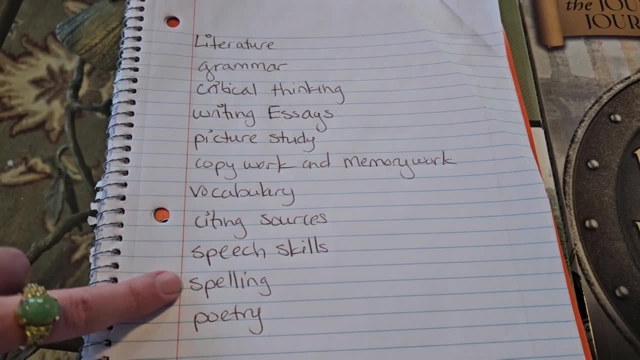 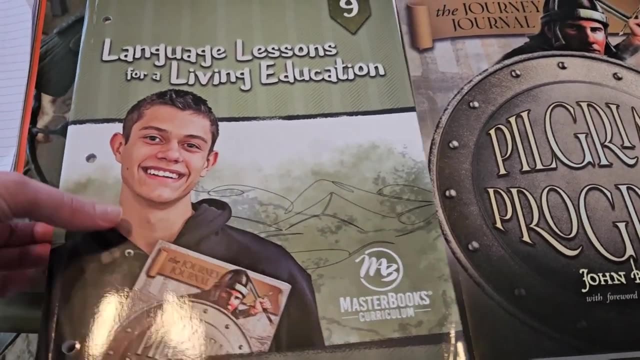 we're probably not going to use the spelling component of it, because he is really good at spelling already And I feel like he gets plenty of that from the copywork. There are two books that it comes with: The main textbook and the Pilgrim's Progress. This is the Journey Journal. 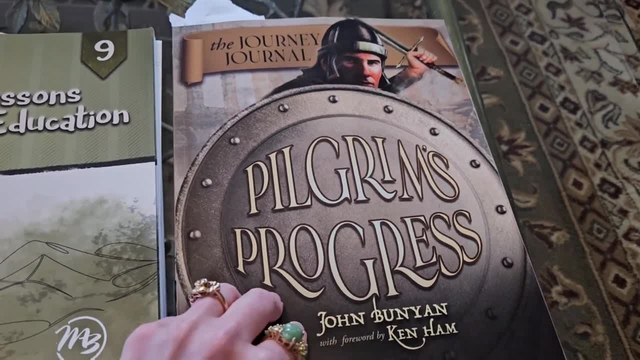 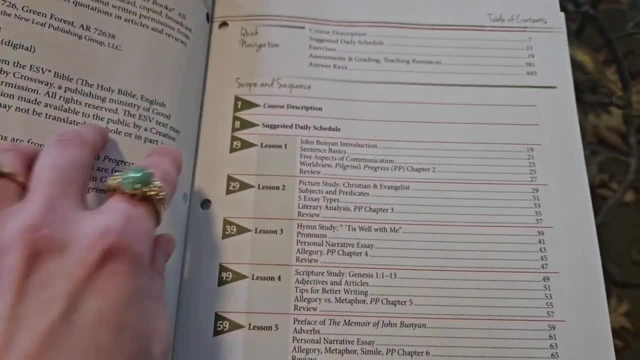 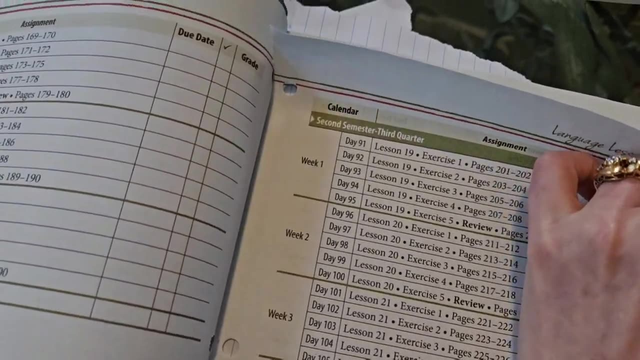 and this is published by Master Books. It's a little bit different than just reading from the regular Pilgrim's Progress book. So this is the main textbook. I just want to bring up that. the pages are really really easy to rip out from here. They're perforated and they just come out. 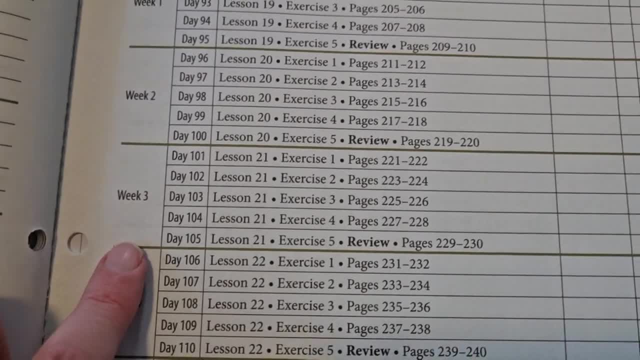 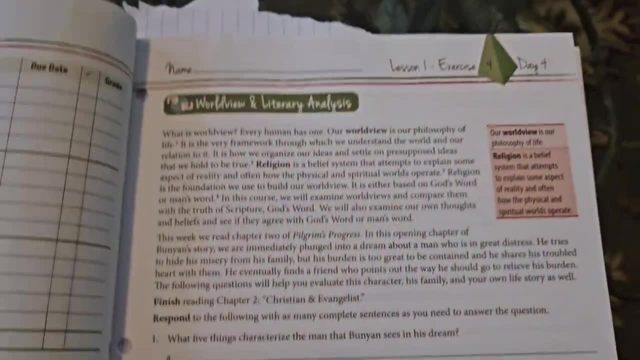 easily. There is a schedule to follow in the very beginning. I don't think this is completely necessary, because everything is clearly marked out for which pages you have to do in the lessons themselves. Let me show you, guys, a week of work in this book. I'm going to show you a week of work. 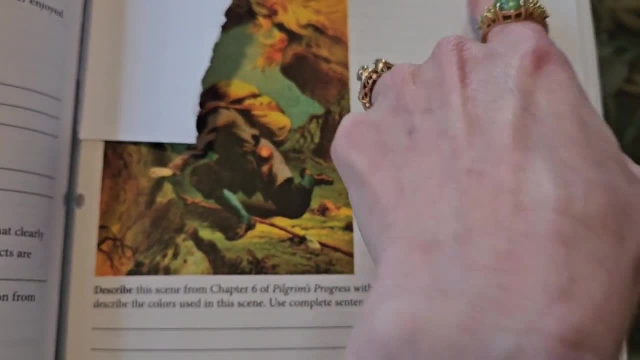 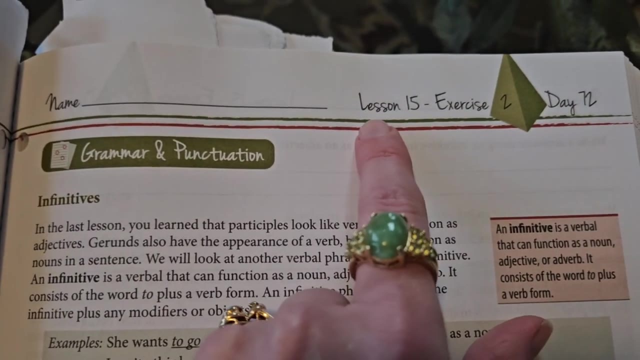 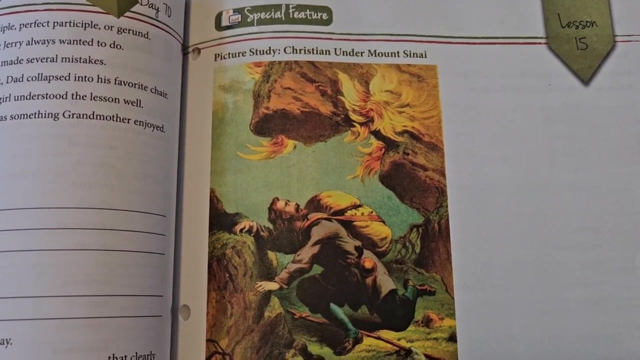 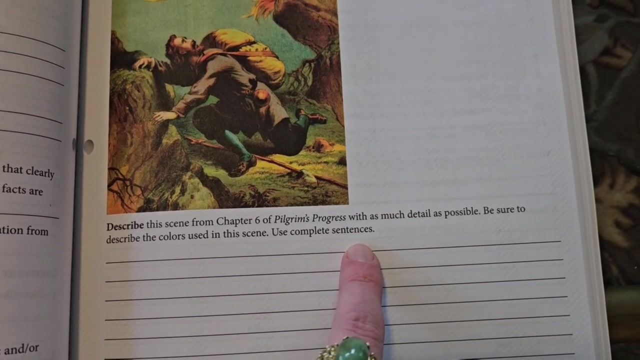 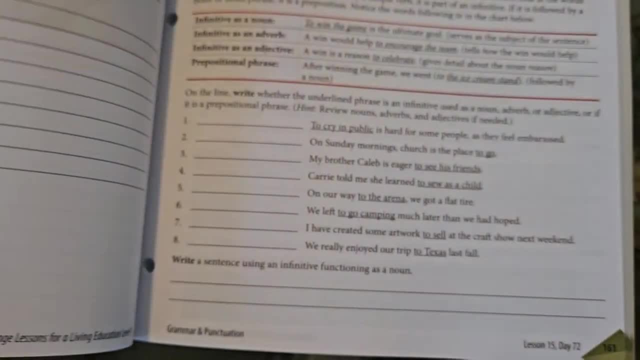 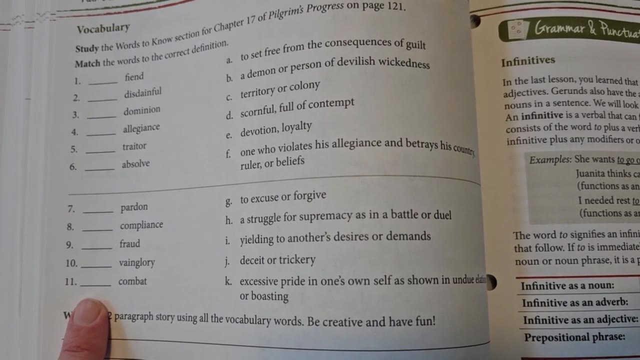 He doesn't like to hand write a lot of stuff, so he'll probably type this up. And then usually day one you'll go into the vocabulary work, which the vocabulary is straight from the Pilgrim's Progress story, And then over here there's activity for vocabulary. 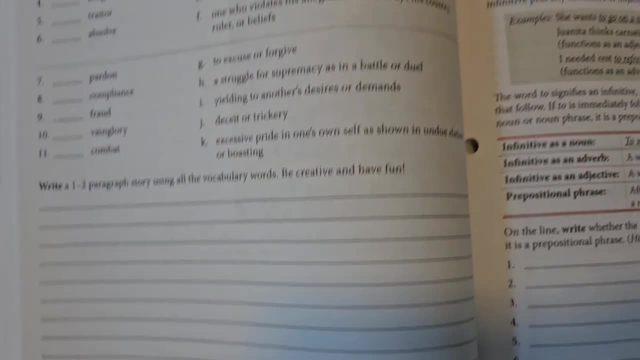 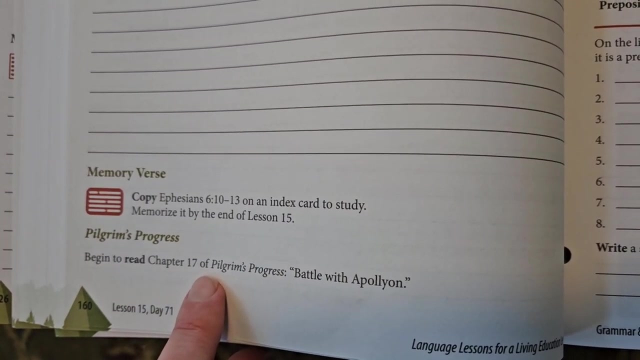 Write one to two paragraph story using all the vocabulary words. There's copy work And over here it says to read chapter 17 of Pilgrim's Progress. Let me show you what that looks like in the book here of Pilgrim's Progress Journal. 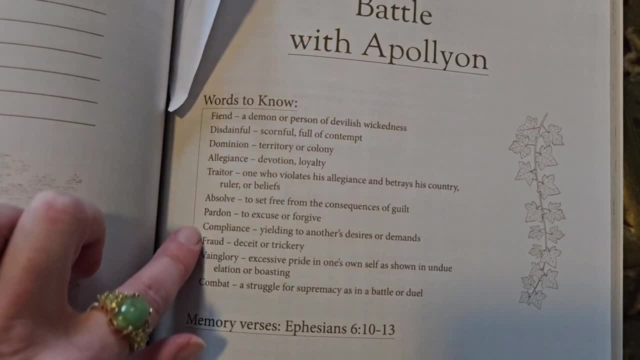 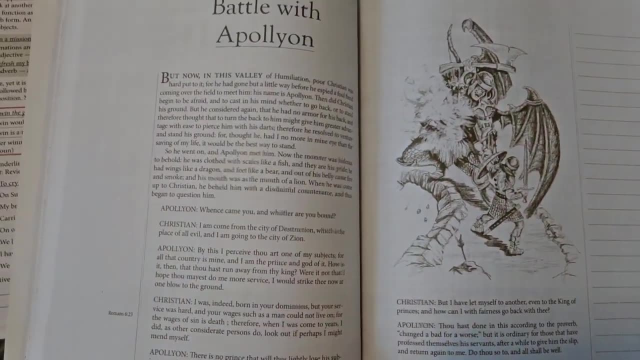 Chapter 17.. These are the same vocabulary words that you saw in the lesson. Here's the memory verse that were from the lesson in the main textbook And then you go into the chapter reading. There's not a whole lot of reading and I know my son's going to be able to finish this in one day. 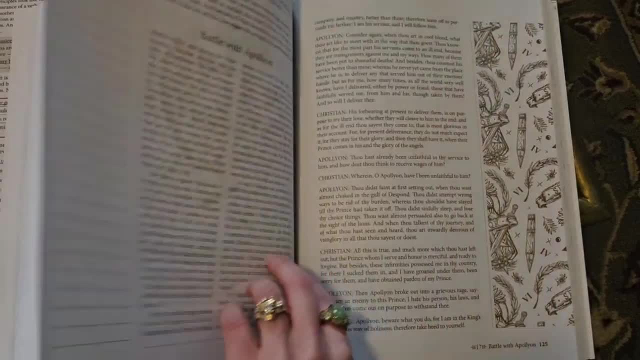 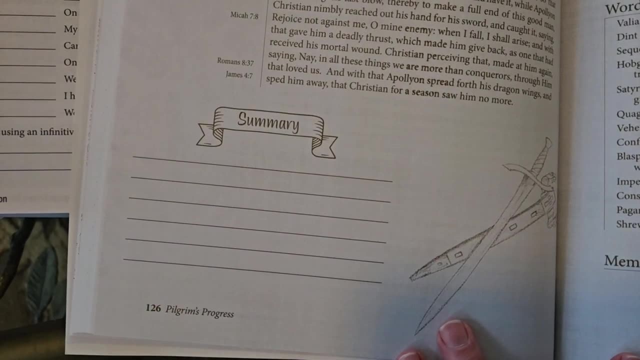 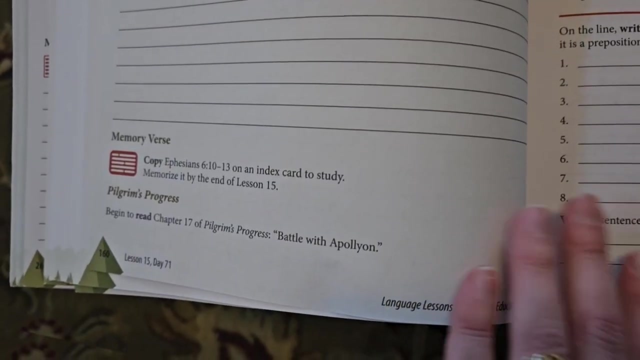 So this is Just one chapter, Just a few pages, And that's the end of the chapter already there, And then there's a spot for a summary at the end of it. So that was just day one of lesson 15, or week 15.. 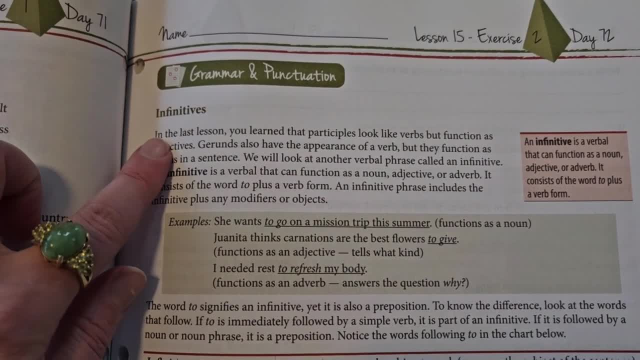 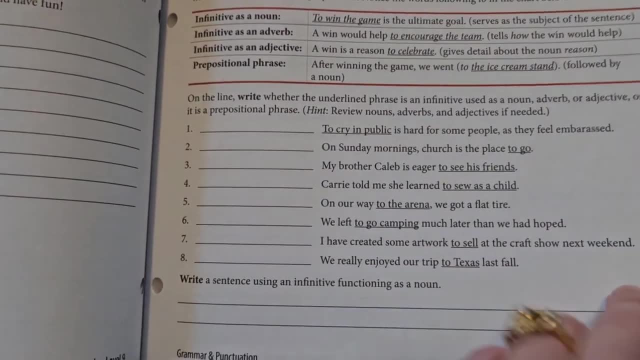 Day two goes into grammar and punctuation. This is infinitives for the lesson. It goes into a nice explanation about them And then it has activities And there's more writing here. It always says to write in complete sentences, which is more writing practice. 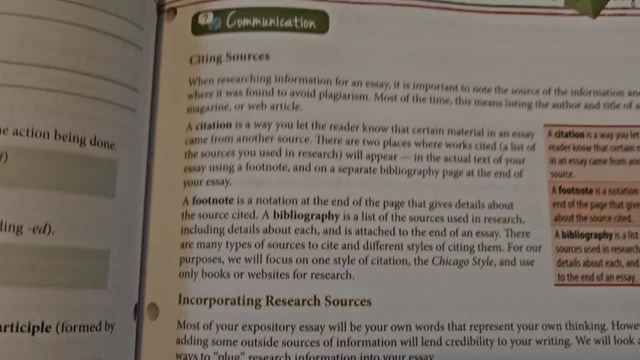 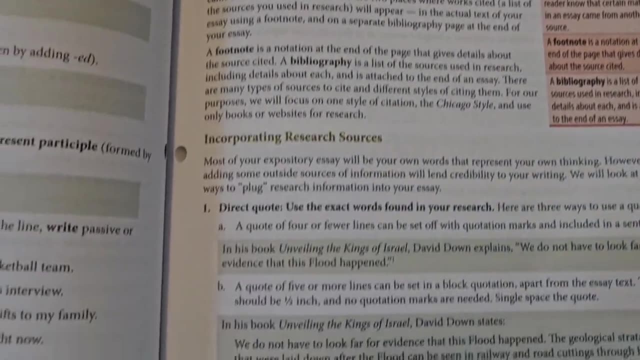 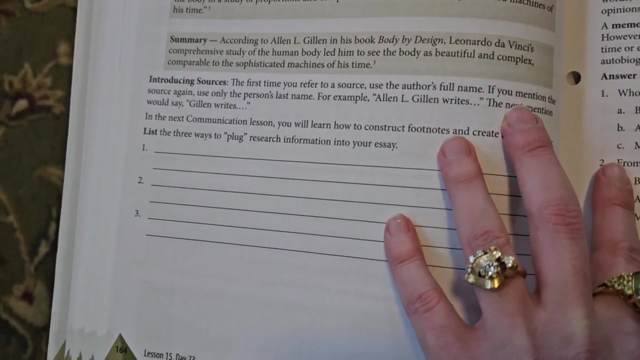 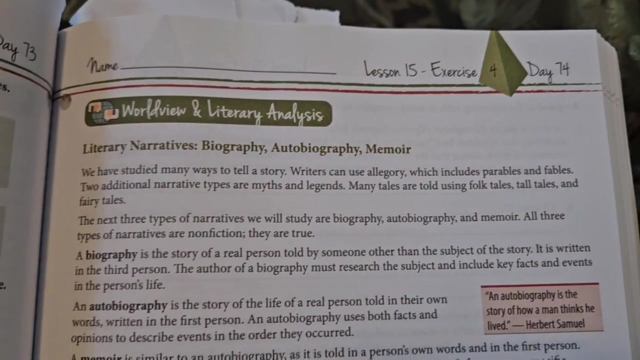 There's more activities And then the next day, lesson 15, exercise 3, day 73.. It goes into citing sources And all of these lessons are pretty much two pages long, So it's very easy to follow along. Then next page, lesson 15, exercise 4, day 74.. 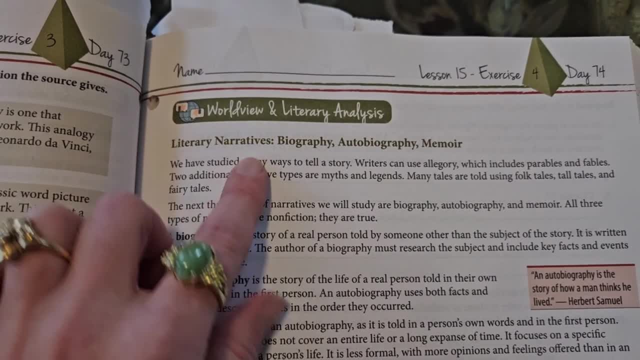 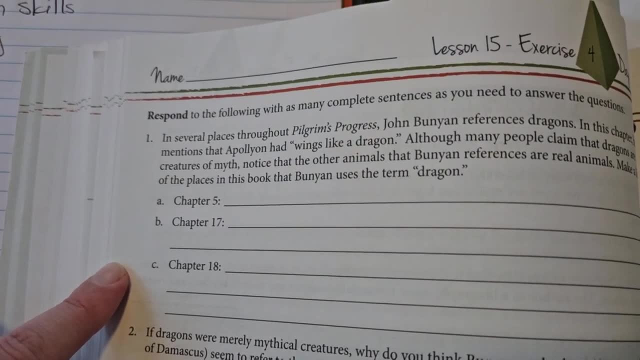 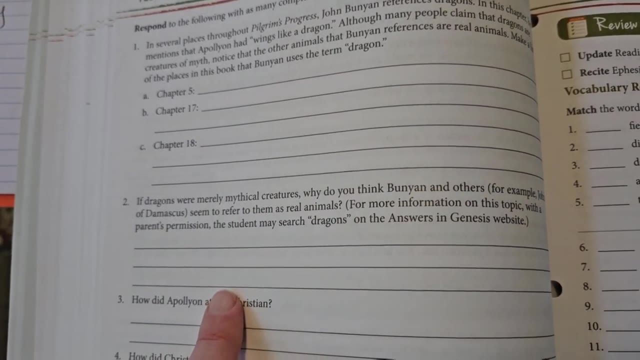 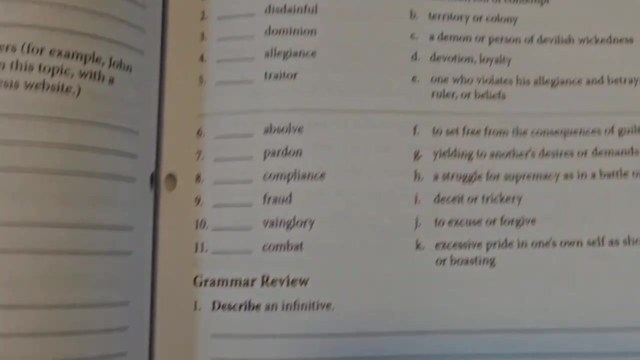 Literary narratives, biography, autobiography and memoirs. That's what this lesson is about. It says: respond in complete sentences again. Little things like this he'll probably just handwrite, but bigger sections he'll be typing up. And then day 5, or exercise 5, is always going to be a review for what they learned throughout the week. 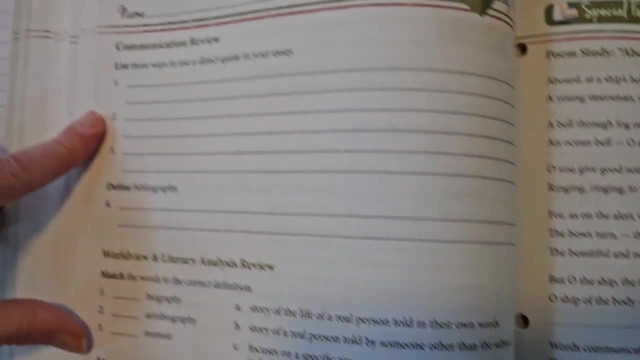 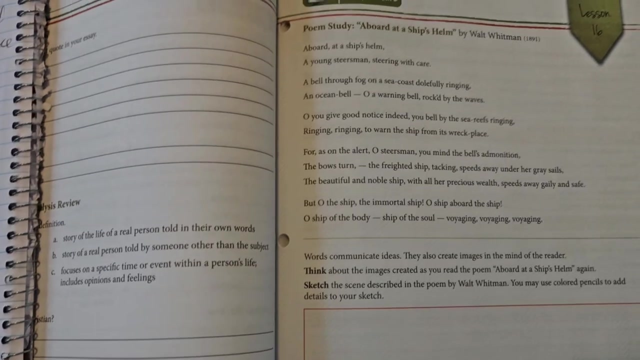 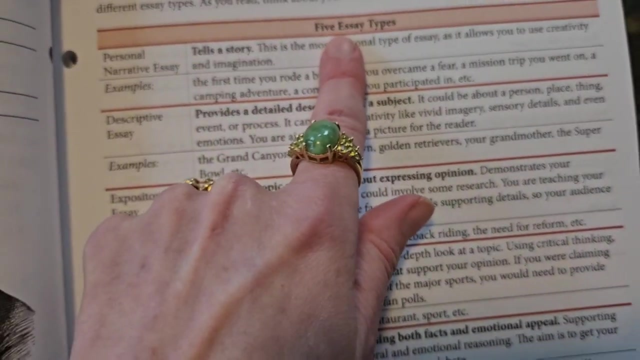 There's grammar review. So some other things I want to go into are different types of papers they're going to be writing throughout the year. I believe they're going to be writing all of these papers. It goes into five essay types: Personal narrative. 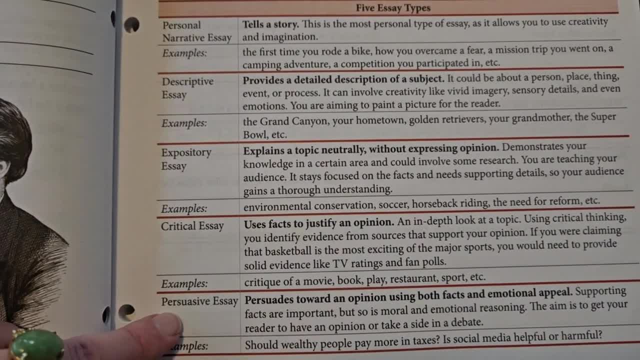 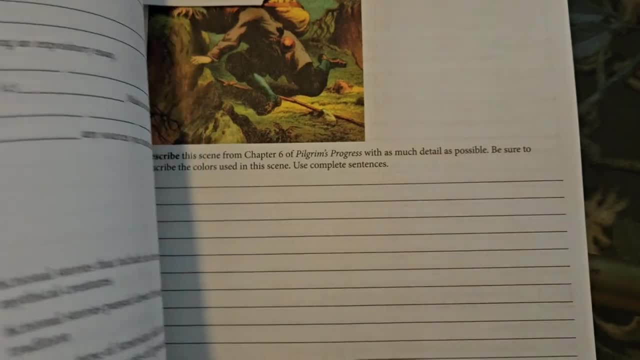 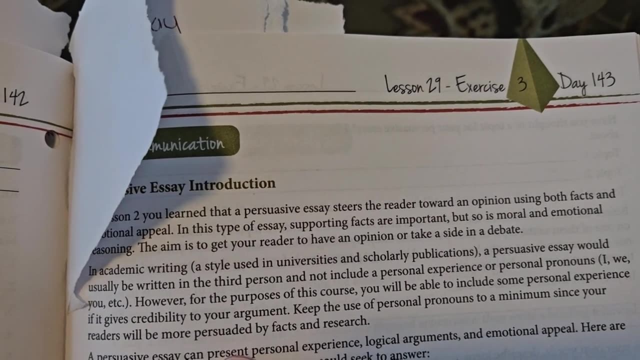 Descriptive expository, critical essay and persuasive essay. I'm pretty sure they're going to end up writing a paper for all of those throughout the year. And let me show you the section on persuasive essay. It's lesson 29,, exercise 3, day 143.. 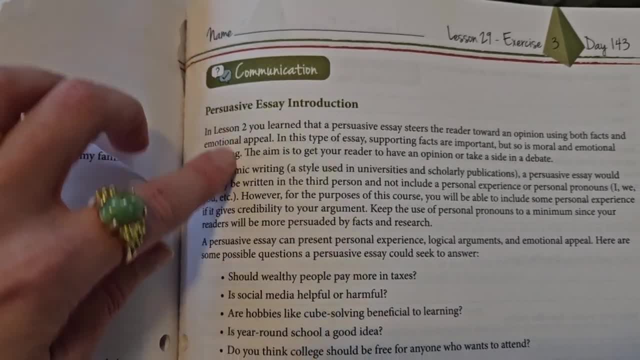 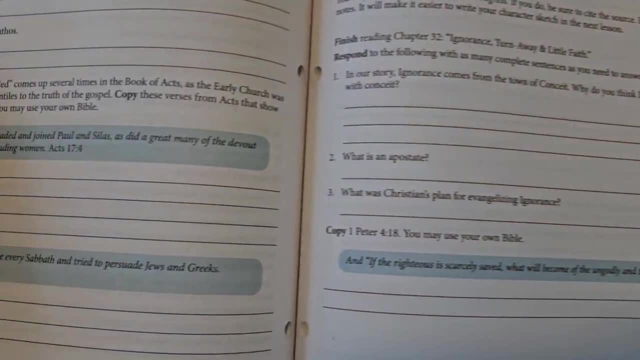 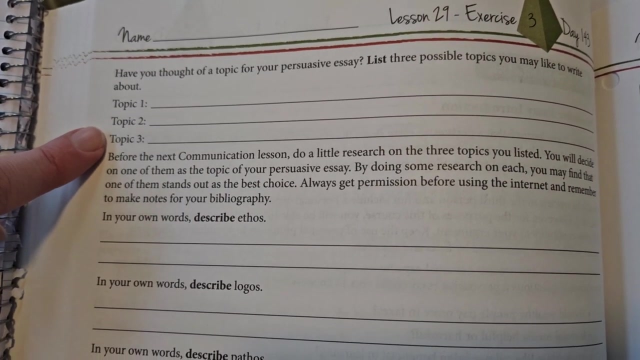 It goes into an introduction about persuasive essays, Which is really good that it breaks it down this much for them. It's giving them so much detail And then they have to do some activities on it. Over here they have to come up with three ideas for an essay. 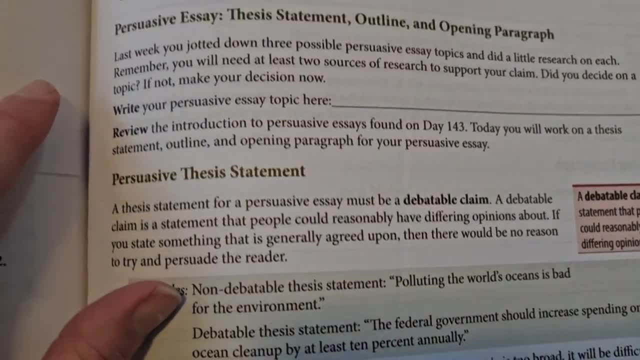 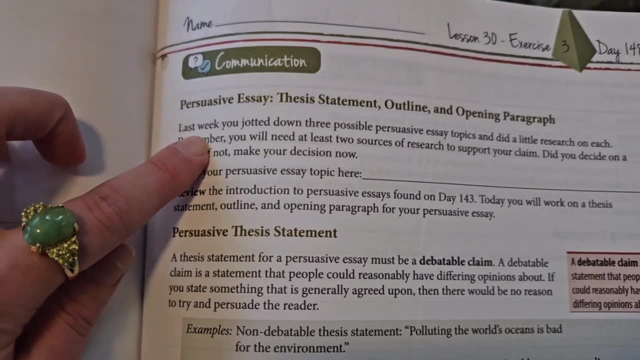 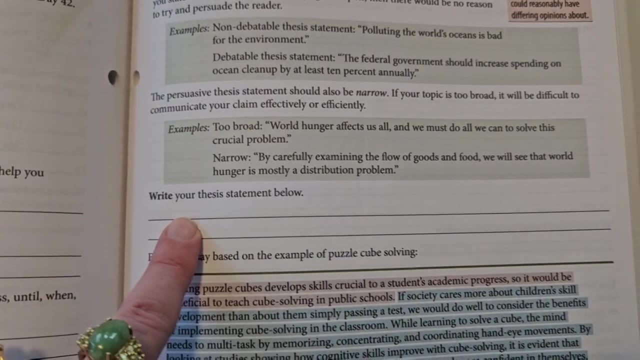 And then the next week they actually start writing the essay. So this is going to be lesson 30, exercise 3, day 148.. It talks about the thesis statement. It's so great that it breaks it down like this, And then they have to write their thesis statement below. 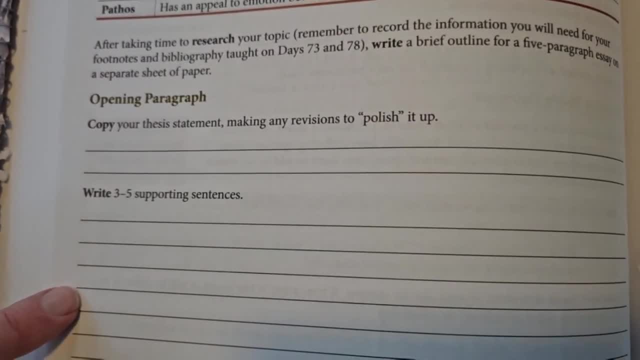 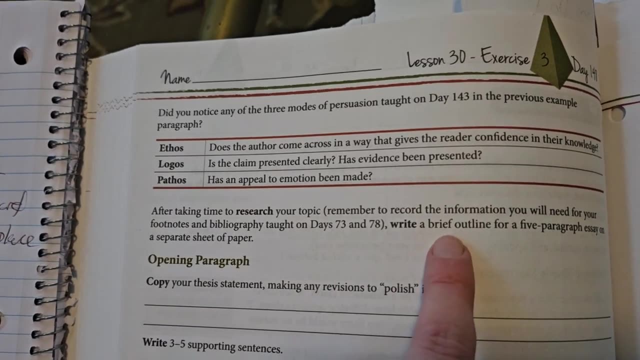 And then And over here they have to write the opening paragraph, the supporting sentences and the concluding paragraph. Okay, so this part over here it tells them to write a brief outline for a five paragraph essay, If your child's already really proficient about writing five paragraph essays. 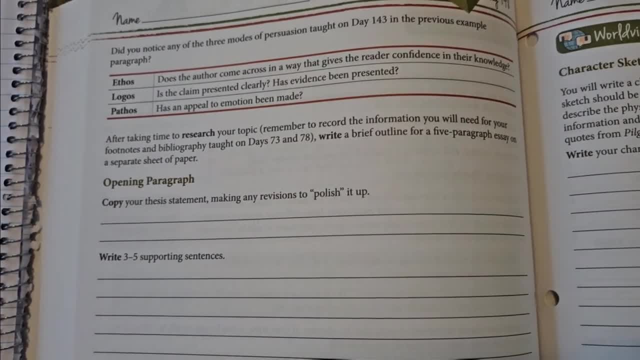 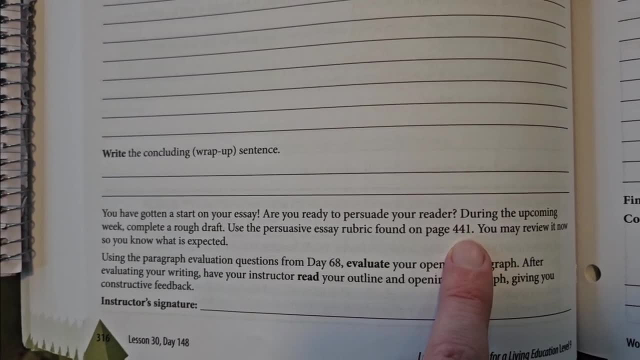 you could always make this a little bit larger and add a few more paragraphs into the middle of it. And then down here it says there is a rubric on page 441.. So they know exactly what they're supposed to be putting into their essay. And it gives them about one week to write a brief outline. And it gives them about one week to write a brief outline, And it gives them about one week to write a brief outline. So it takes about one week to finish this and after that one week. 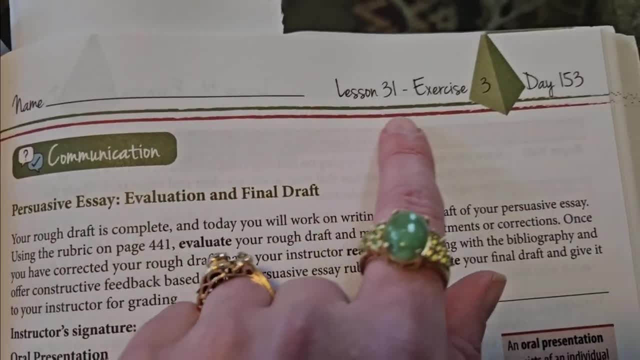 So it takes about one week to finish this, and after that one week There's. So this is lesson 31,, exercise 3, day 153.. So this is lesson 31,, exercise 3, day 153.. So this is lesson 31,, exercise 3, day 153. 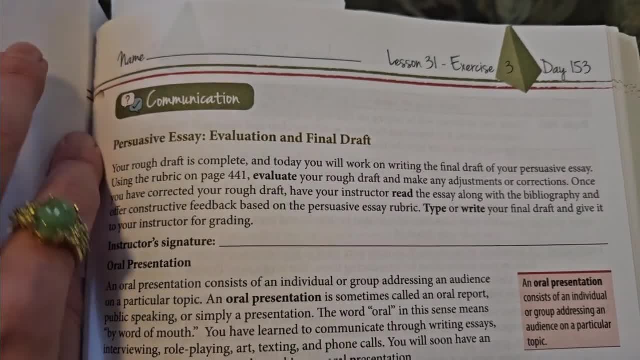 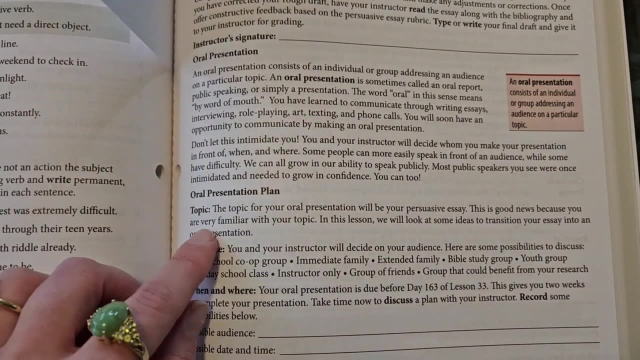 It's persuasive essay evaluation final draft. So they would be going into the rubric, they would be fixing it up And they would be doing their final draft at this point. It's really nice that it's giving him this many days to write an essay so they can really think about what they're doing. 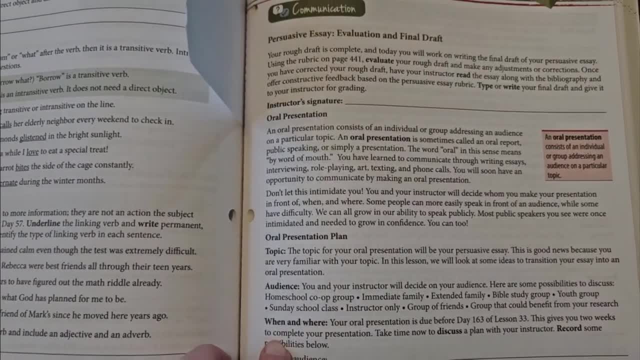 When my older son had completed the EZPZ Literature and Composition when he was in 9th grade. it moved a lot quicker than before. It completed the Easy Peasy Literature and Composition When he was in 9th grade. it moved a lot quicker. 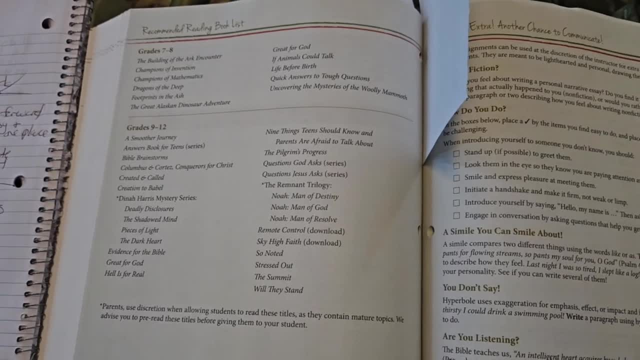 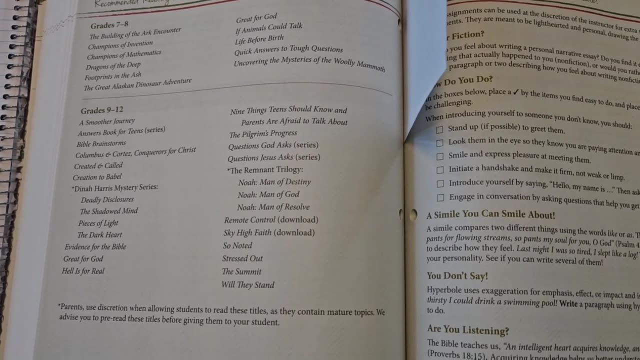 and it didn't give him this many days to work on a paper. So there is a recommended reading list in the back. I'm not going to be using this. We're going to be pulling all of our literature from the Guest Hollow, which is one of the reasons I went with this program. 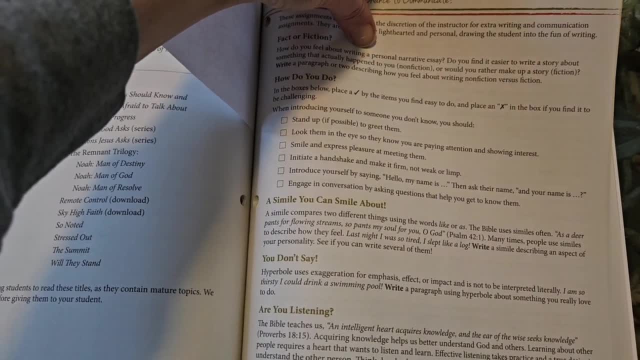 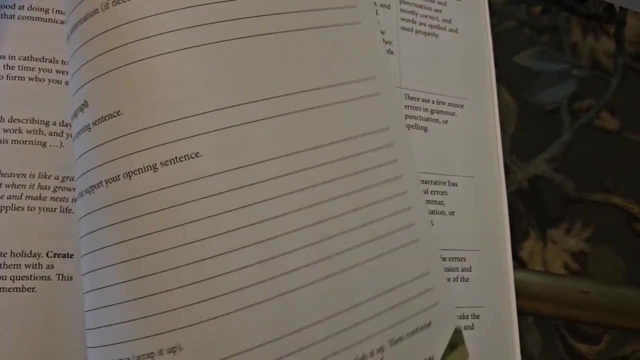 I always had trouble juggling which literature to use- the one from the Easy Peasy or the one from the Guest Hollow- So this is just going to make it easier on me. In the back, here are the rubrics for all the papers we're going to be writing. 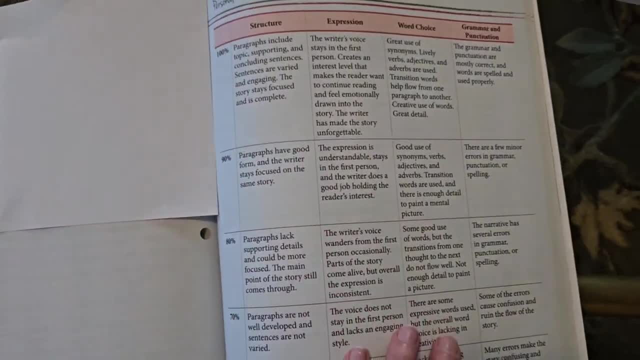 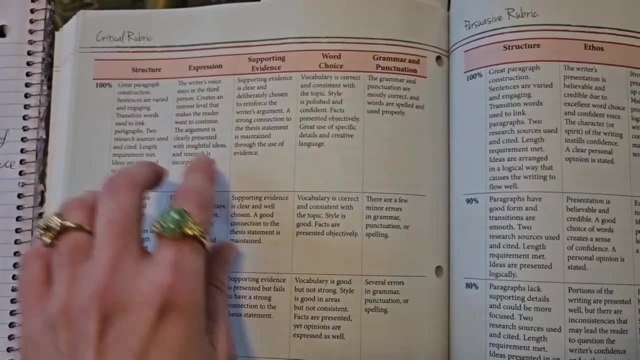 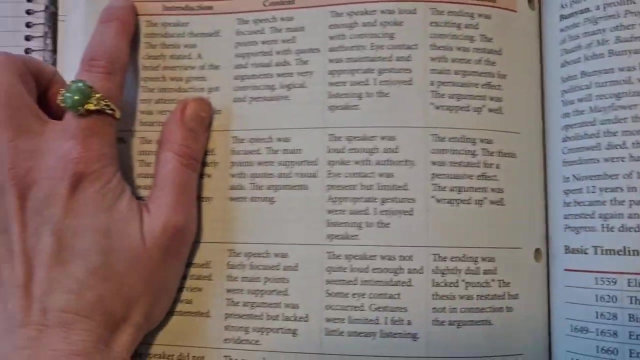 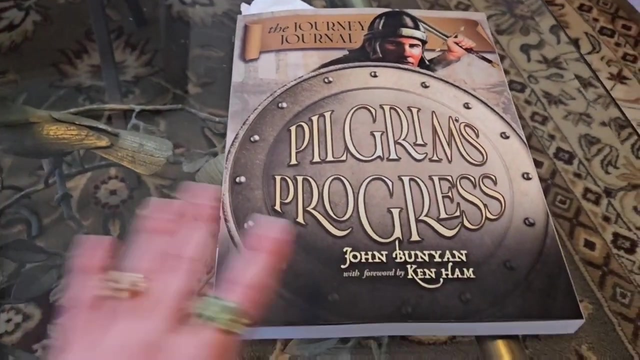 This is for the Personal Narrative rubric. This is the Descriptive. They've gone for Expository. It's the Critical rubric and the Persuasive rubric and the Oral Presentation. So this is where the speech skills come in. All right, I'm going to go over the Pilgrim's Progress Journey Journal right now. 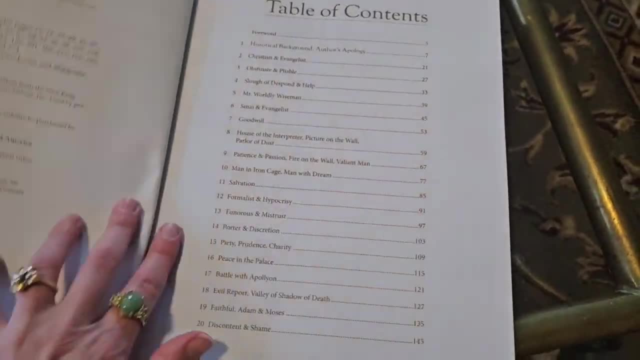 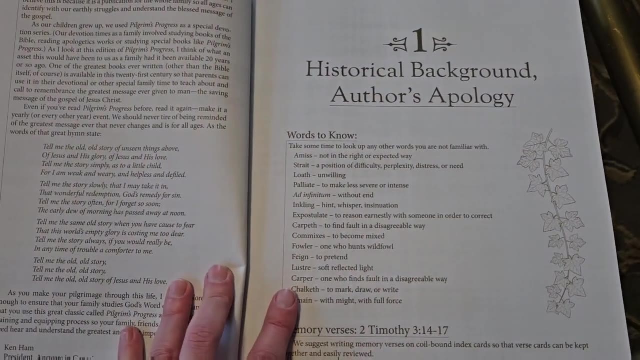 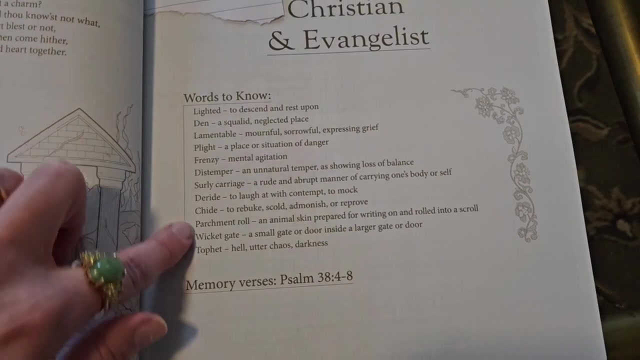 This is printed just by Master Books, just for this curriculum. You start with the Table of Contents, then the Foreword, And Chapter 1 is actually skipped in the curriculum. You jump straight into Chapter 2. And of course each chapter has all the vocabulary words and the memory verse.